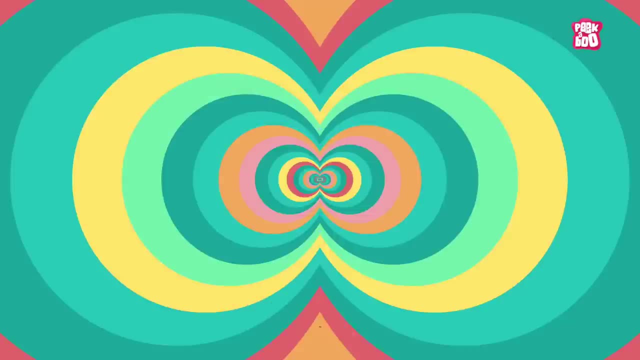 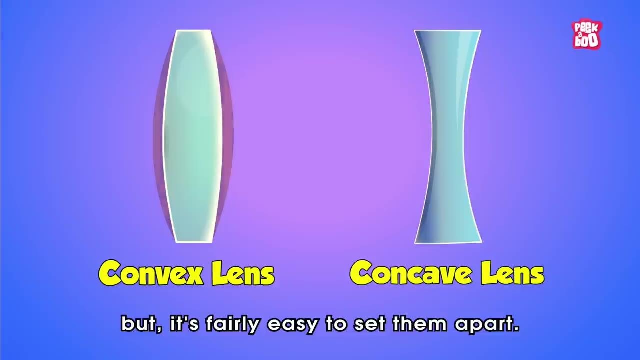 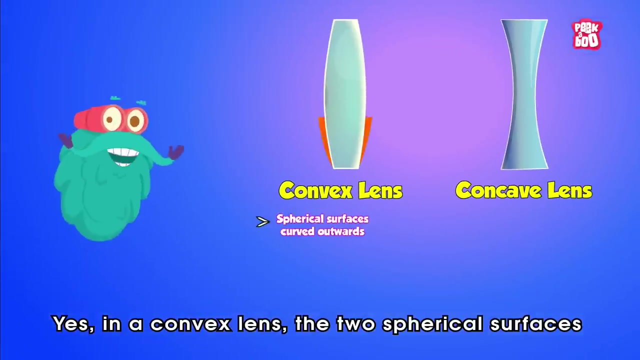 Convex lens and concave lens, Though both the lenses are bordered by two transparent spherical surfaces, but it's fairly easy to set them apart. Yes, in a convex lens the two spherical surfaces meet. The two surfaces are curved outwards, while in the case of a concave lens they are curved inwards. 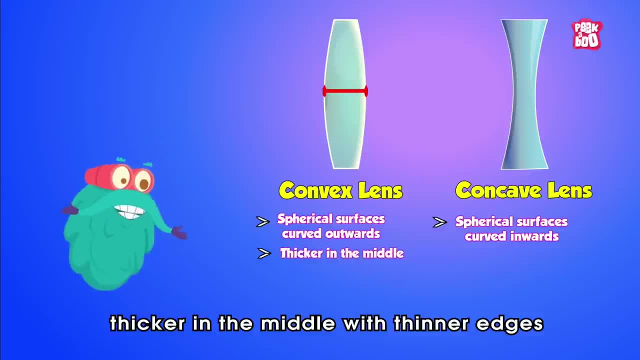 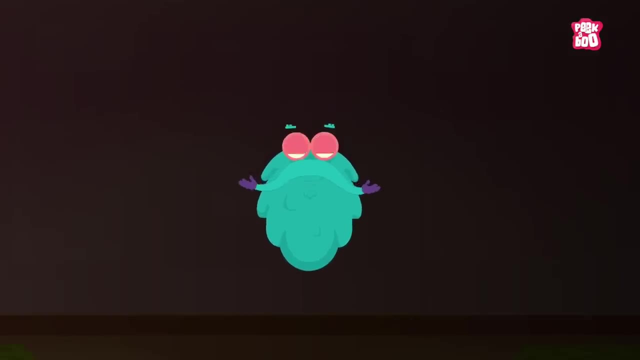 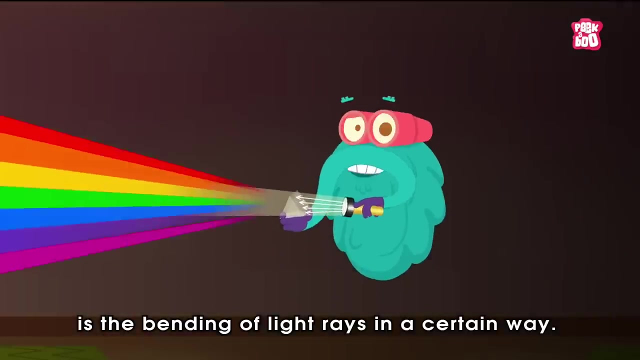 Also, a convex lens is thicker in the middle with thinner edges, while the concave lens has a thin center with thick edges. But the vital question is: how do these lenses work? Well, it's due to refraction, which, as we learned before, is the bending of light rays in a certain way. 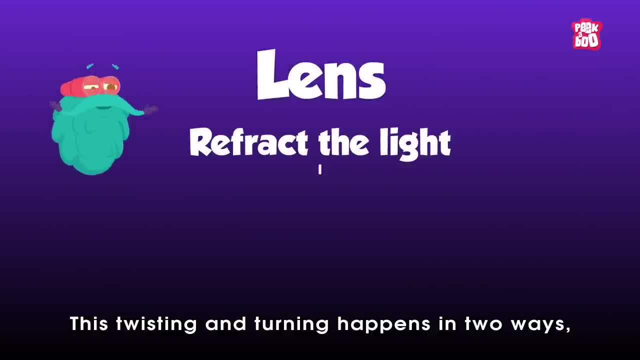 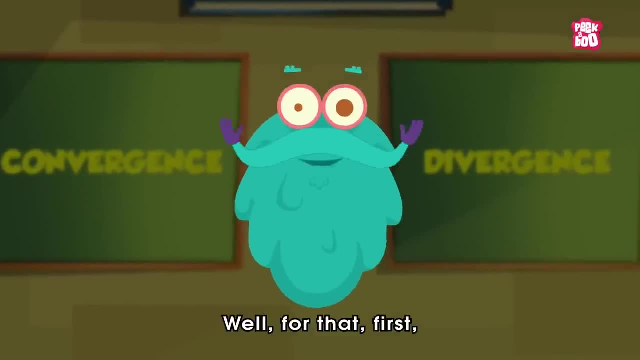 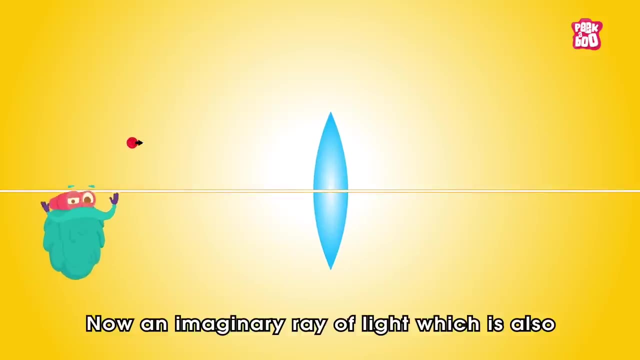 This twisting and turning happens in two ways: convergence and divergence. And what do they mean? Well, for that, first, we must look into the way both the lenses work. Now an imaginary ray of light, which is also called an image ray. 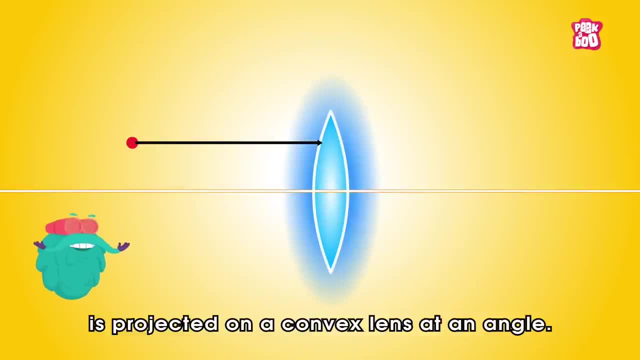 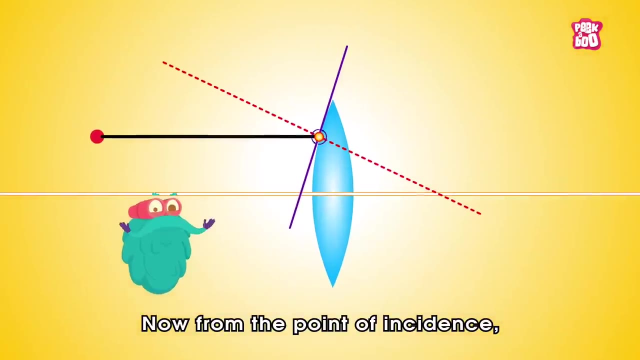 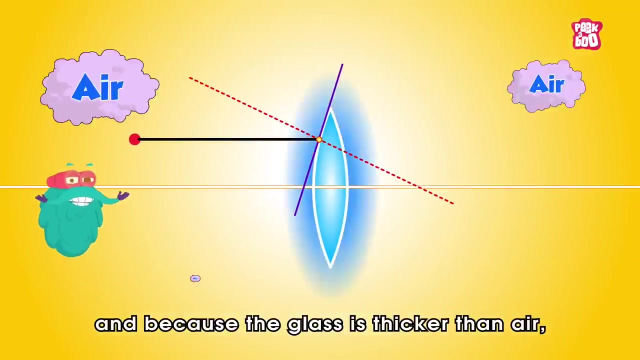 An incident ray is projected on a convex lens at an angle. Then, from the point of the incidence, which is the touching point of the ray and lens, we draw a line known as normal. Now, from the point of incidence, this ray of light will enter the lens and because the glass is thicker than air, 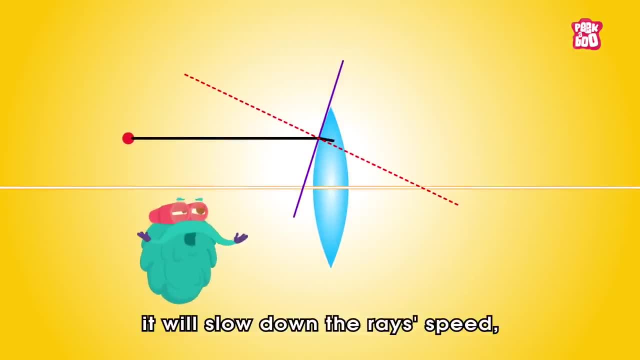 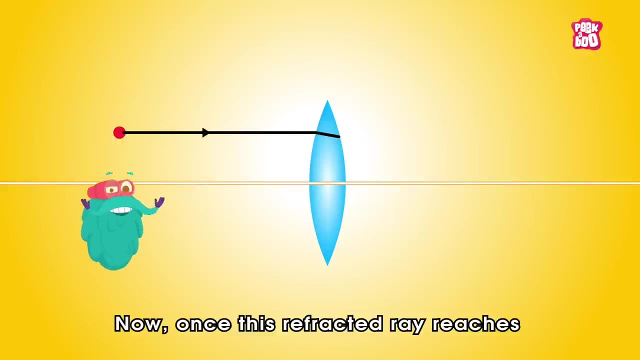 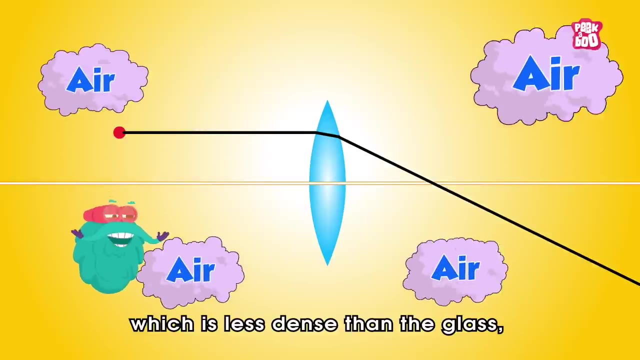 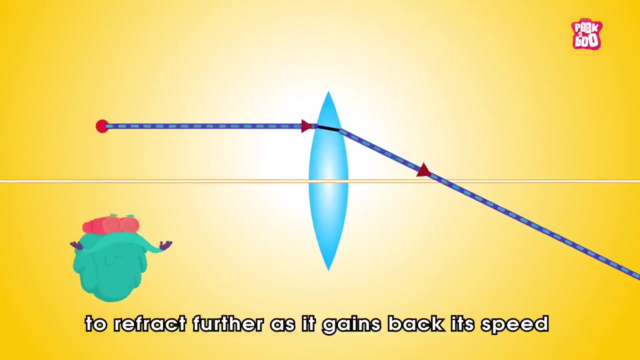 it will slow down the ray's speed and bend it down towards the normal line. Now, once this refracted ray reaches the other surface of the lens and enters the air again, which is less dense than the glass, the momentum pushes the light to continue to refract further as it gains back its speed. 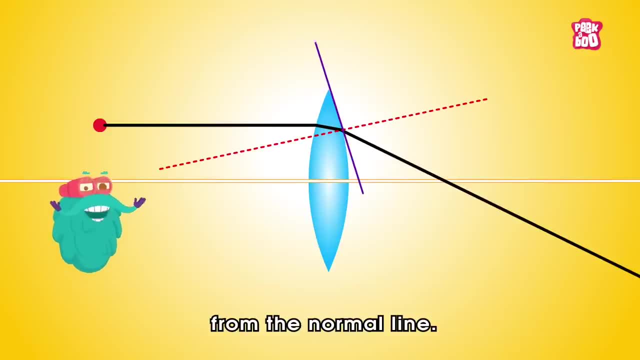 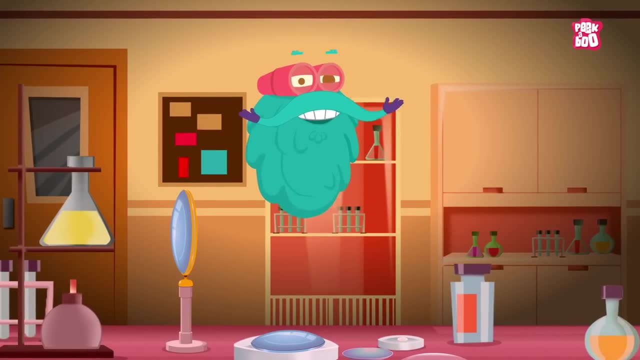 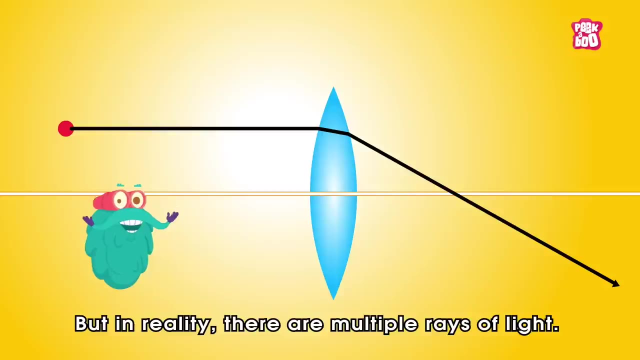 And this time it bends away from the normal line. So, in short, that's how light is refracted by a convex lens. Over here we saw how a single incident light will act in such a scenario, But in reality there are multiple rays of light. 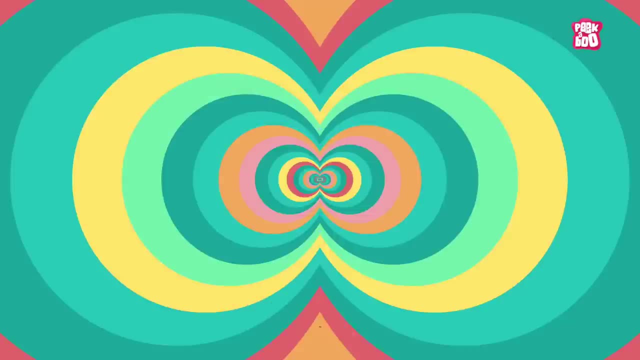 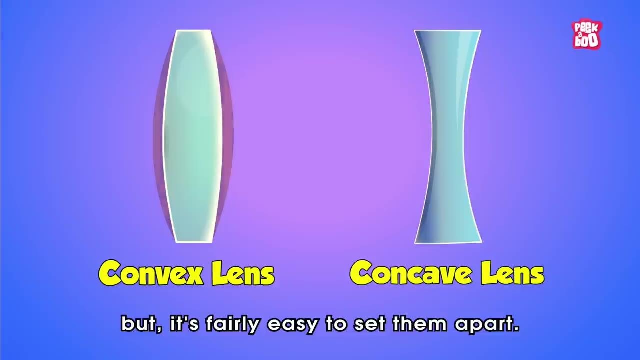 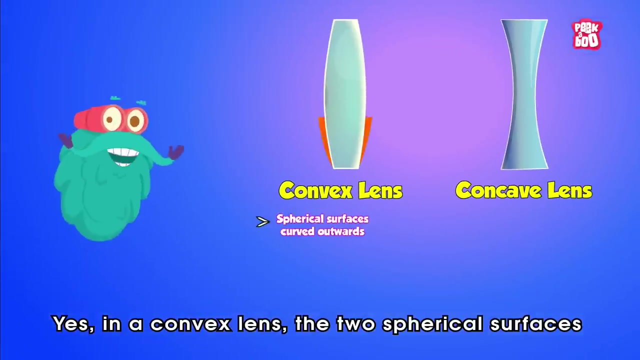 Convex lens and concave lens, Though both the lenses are bordered by two transparent spherical surfaces, but it's fairly easy to set them apart. Yes, in a convex lens the two spherical surfaces meet. The two surfaces are curved outwards, while in the case of a concave lens they are curved inwards. 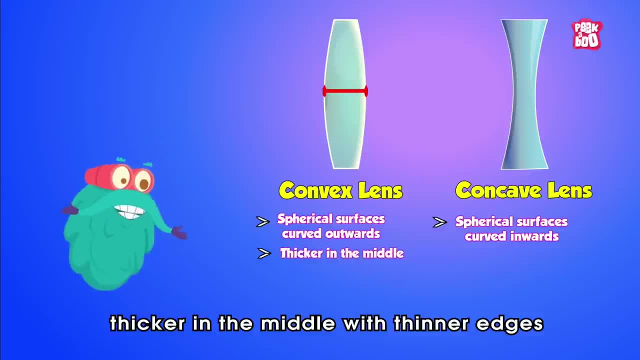 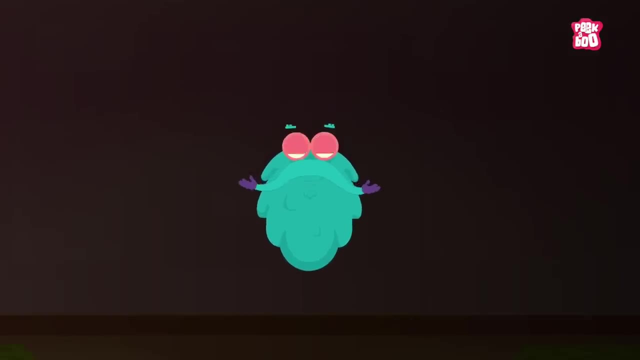 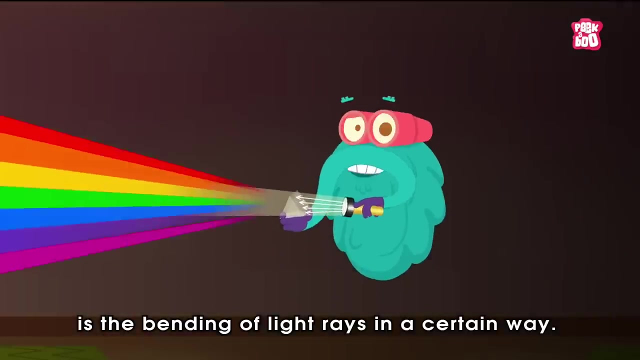 Also, a convex lens is thicker in the middle with thinner edges, while the concave lens has a thin center with thick edges. But the vital question is: how do these lenses work? Well, it's due to refraction, which, as we learned before, is the bending of light rays in a certain way. 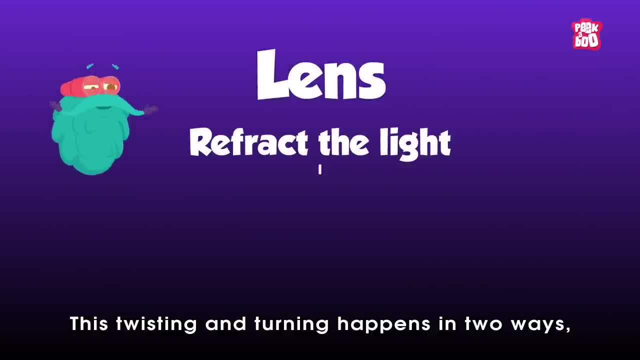 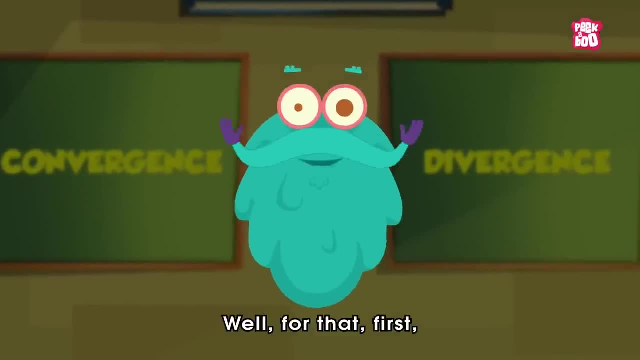 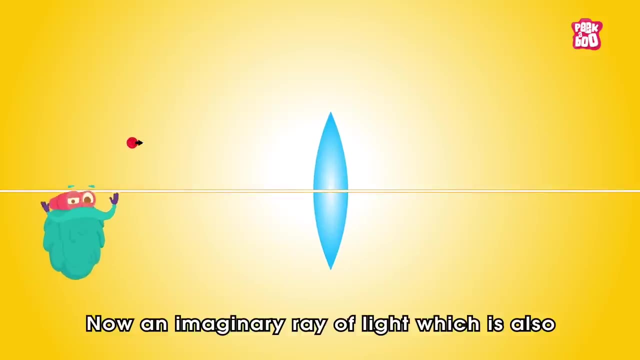 This twisting and turning happens in two ways: convergence and divergence. And what do they mean? Well, for that, first, we must look into the way both the lenses work. Now an imaginary ray of light, which is also called an image ray. 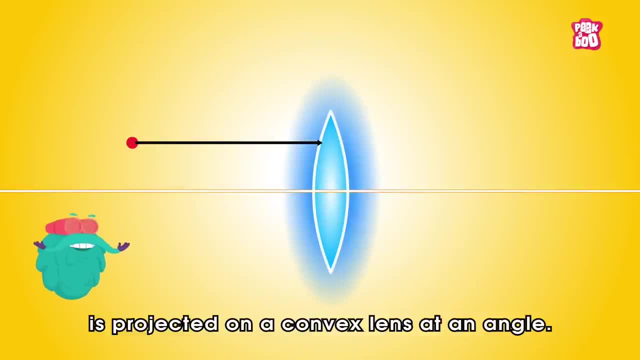 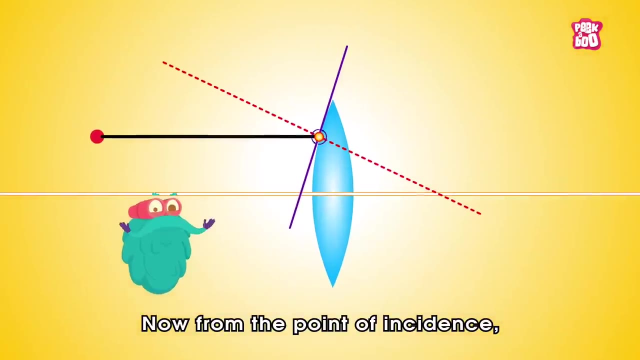 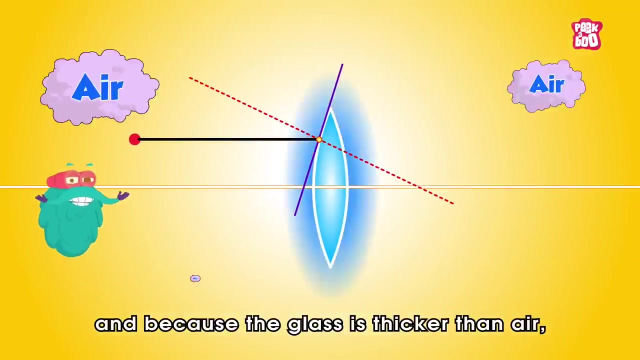 An incident ray is projected on a convex lens at an angle. Then, from the point of the incidence, which is the touching point of the ray and lens, we draw a line known as normal. Now, from the point of incidence, this ray of light will enter the lens and because the glass is thicker than air, 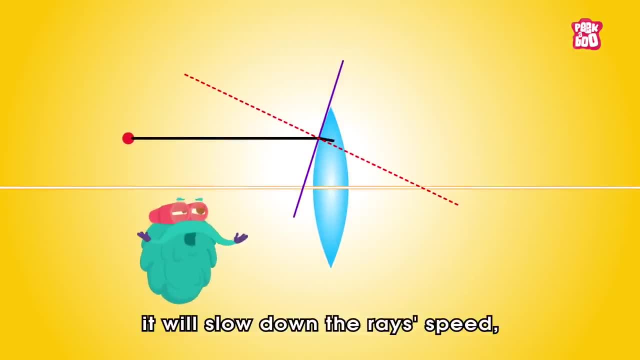 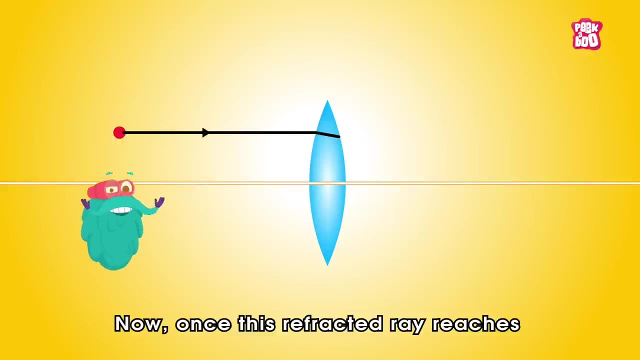 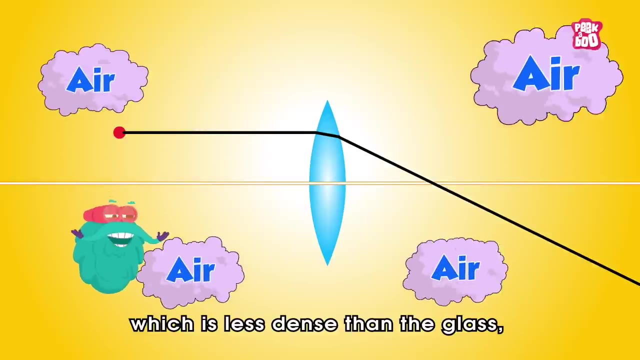 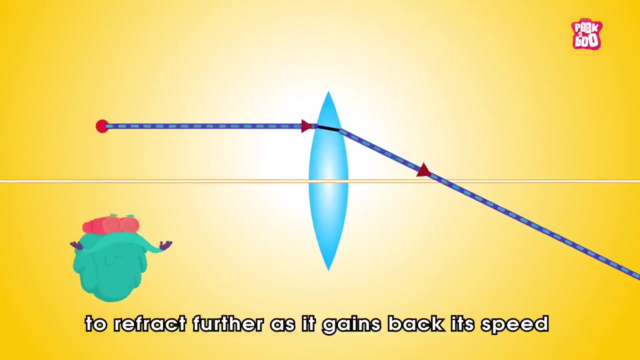 it will slow down the ray's speed and bend it down towards the normal line. Now, once this refracted ray reaches the other surface of the lens and enters the air again, which is less dense than the glass, the momentum pushes the light to continue to refract further as it gains back its speed. 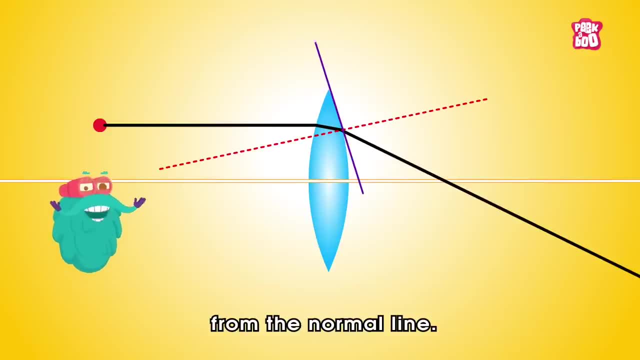 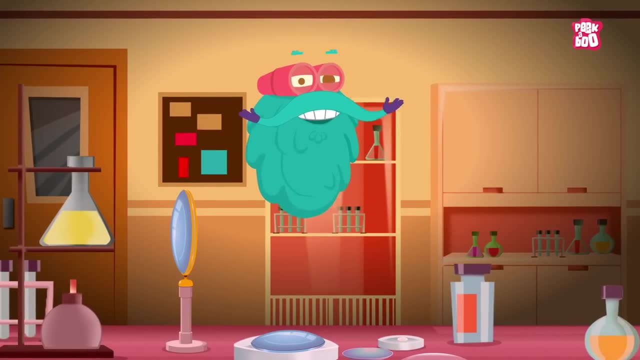 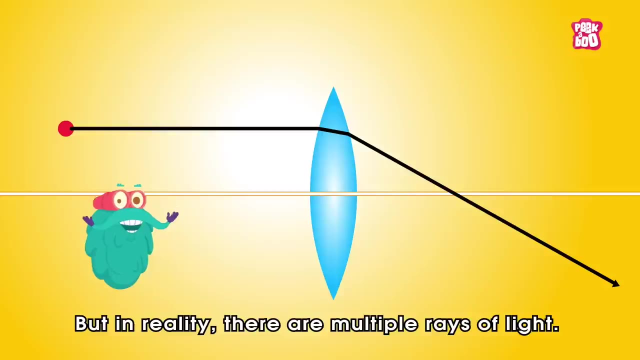 And this time it bends away from the normal line. So, in short, that's how light is refracted by a convex lens. Over here we saw how a single incident light will act in such a scenario, But in reality there are multiple rays of light.